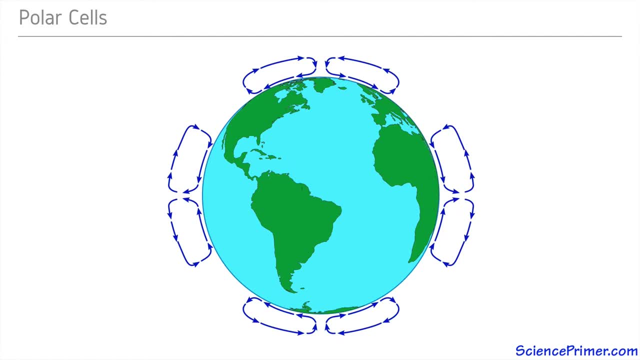 This cell runs to about 60 degrees north and south latitude Before Coriolis. deflection and surface warming cause air to rise, completing the cycle. This is called the polar cell. A third cell exists between the Hadley and polar cells. Air movement here is driven by air that falls along the edge of the Hadley cells but then 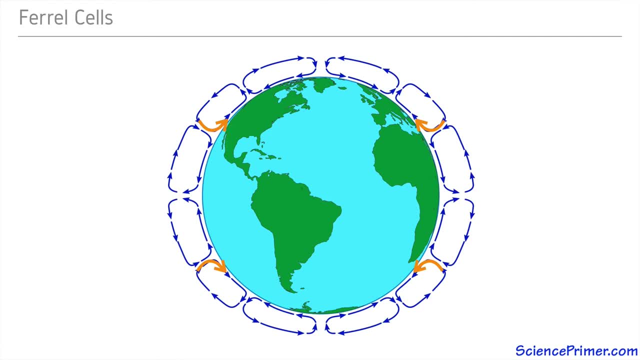 is pushed along the ground away from the equator, and air that rises at the edge of the polar cells that is then pushed back towards the equator. These are called the Farrell cells after the American meteorologist William Farrell. This model of convection cycles diverted by Coriolis effect does a good job capturing. 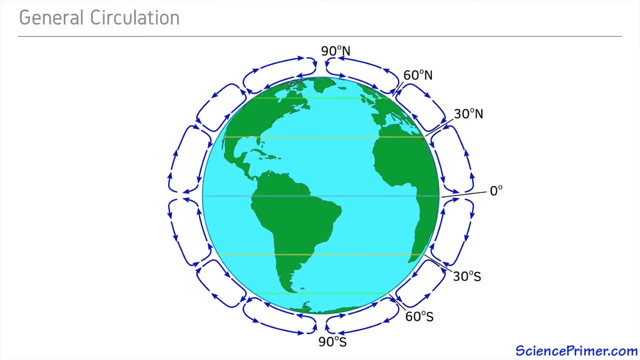 the general characteristics of atmospheric circulation on Earth by explaining the three convection cells on either side of the equator, with alternating regions of high and low pressure between them. The direction of airflow along the ground within each cell creates the prevailing winds found at different latitudes. 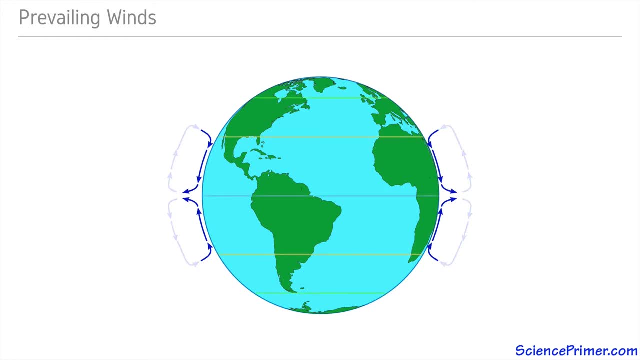 The Hadley cells near the equator move air towards the equator along the ground. Coriolis deflection causes this air to turn to the equator. Coriolis deflection causes this air to turn to the equator. Coriolis deflection causes this air to turn to the equator. 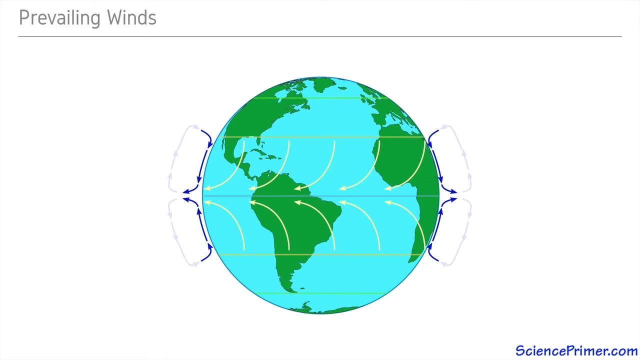 west. Since winds are described by the direction they come from, these are called the easterly trade winds that run between 30 degrees north and 30 degrees south. latitude: Surface air moves away from the equator between 30 and 60 degrees latitude, and the deflection of these currents 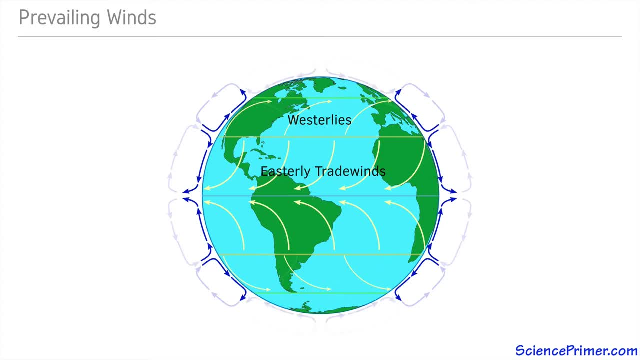 create westerly winds Between the poles and 60 degrees, surface air moves from the poles and is diverted to the west. The location of these high and low pressure systems and the movement of air between has a major impact on precipitation and evaporation Within each of these cells. the low 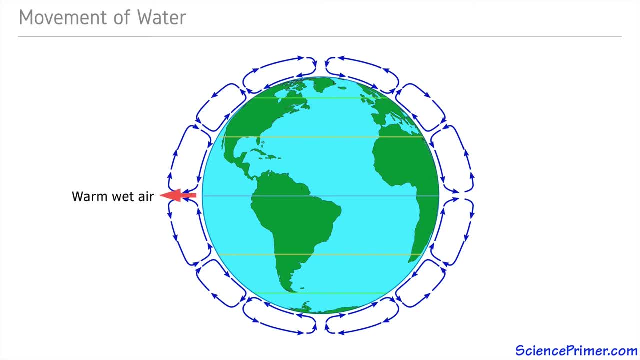 pressure regions move warm water containing air up towards the top of the troposphere. As this air moves away from regions of low pressure, it cools and gives up water vapor, which falls as precipitation At the edge of the convection cells. the now cool, dry air falls, creating regions of 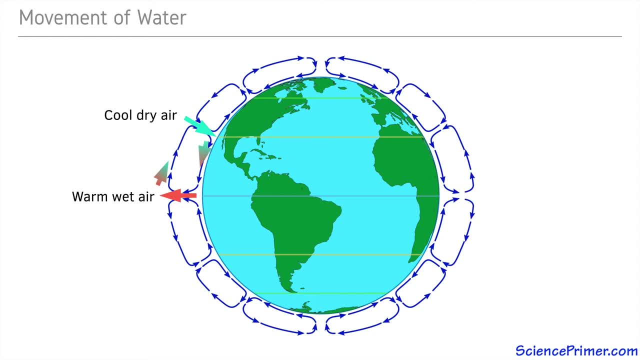 high pressure. Once it reaches the ground, the cool, dry air moves back along the ground, warming and picking up the air. The air moves back along the ground, warming and picking up the air. The air moves back along the ground, warming and picking up water vapor, as it goes This pattern creates.